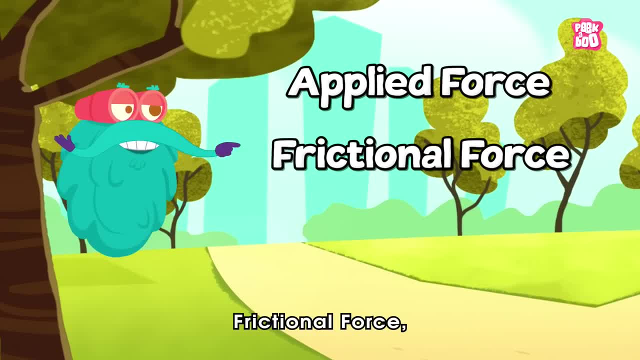 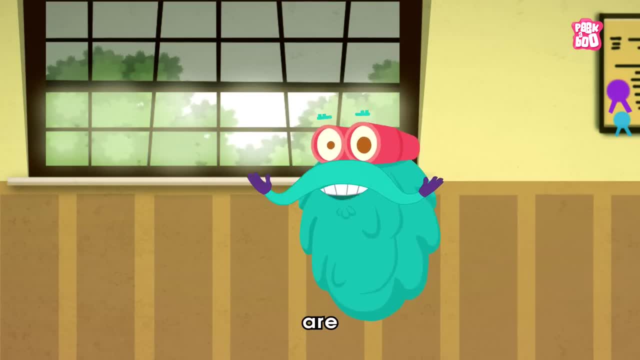 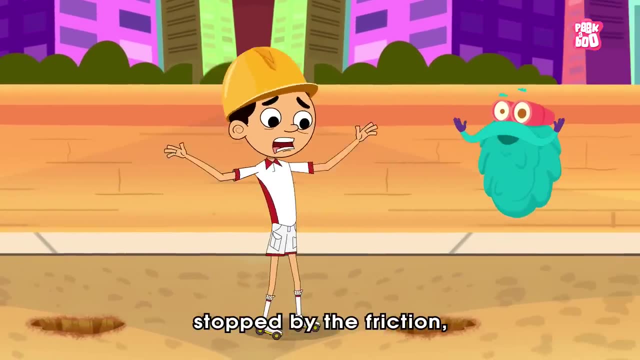 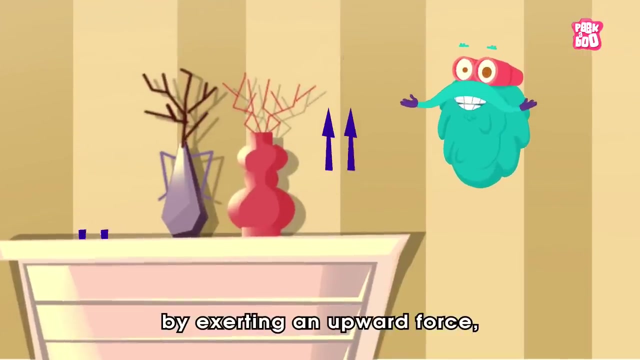 such as applied force, frictional force, normal force, etc. And some of the examples of contact force are: 1. A person pushing a huge wooden box. 2. A person skating on a rough floor stopped by the friction. 3. A table supporting a vase kept on it by exerting an upward force, and much more. 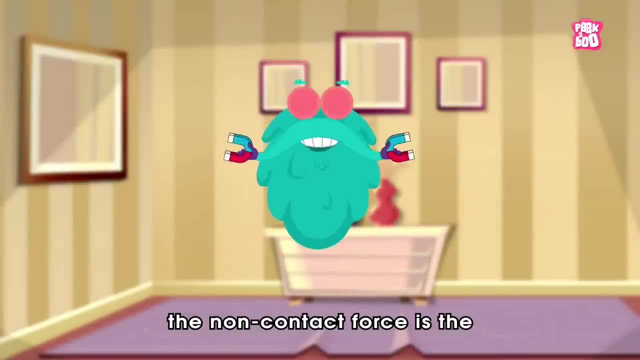 4.. On the other hand, the non-contact force is the opposite of the contact force, meaning during a non-contact force, two objects are in contact with each other. The objects do not come into physical contact with each other during the interaction. The main types of non-contact force are: 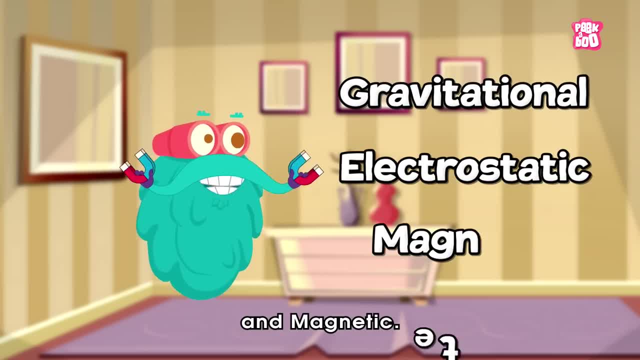 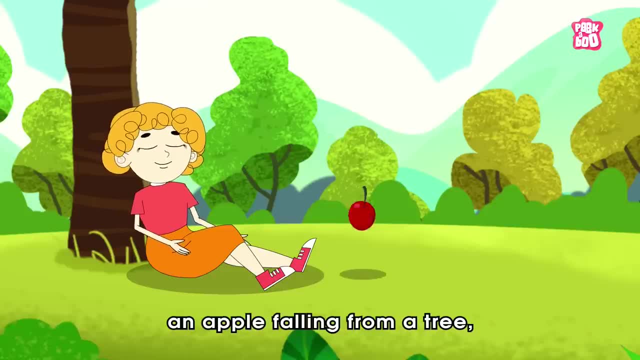 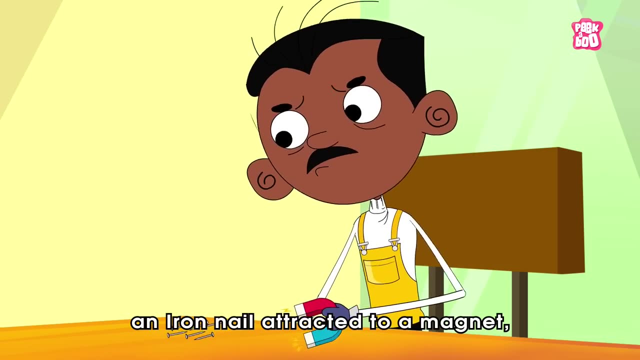 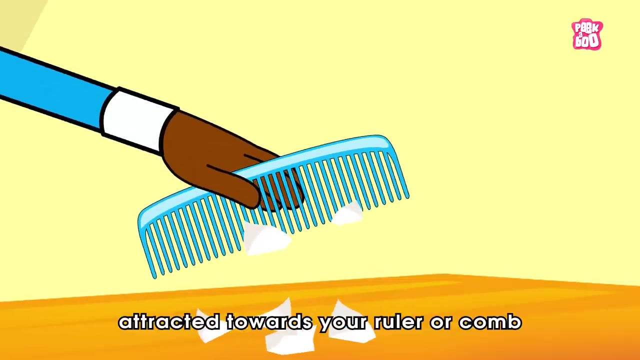 gravitational, electrostatic and magnetic. Some of the examples of non-contact force are: 1. An apple falling from a tree, 2. A football kicked high in the air falling towards earth, 3. An iron nail attracted to a magnet, 4. Pieces of paper attracted towards your ruler or comb when rubbed. 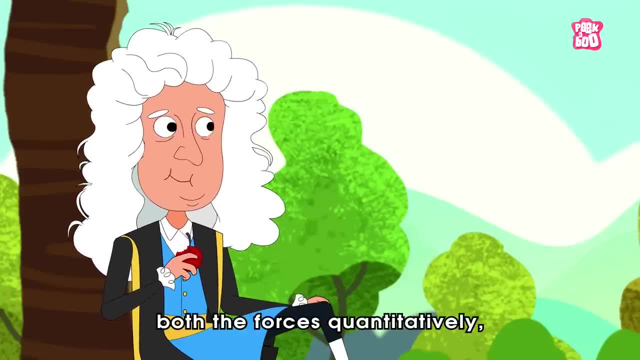 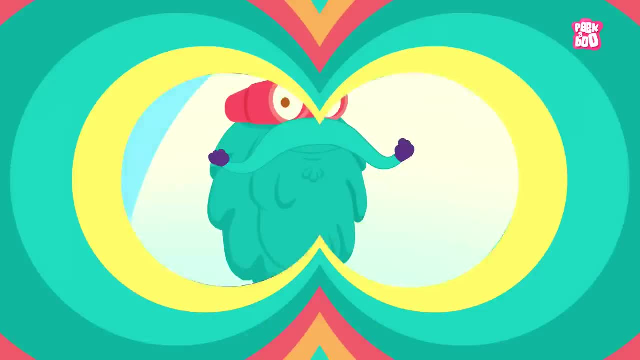 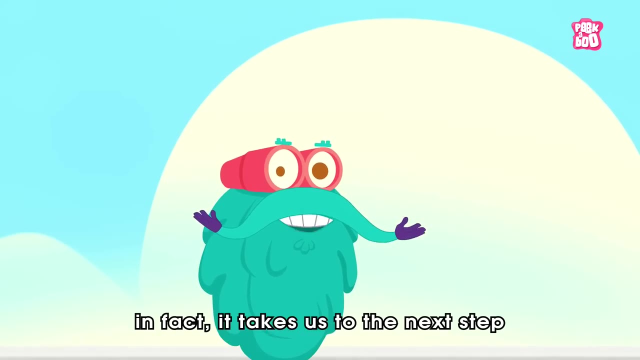 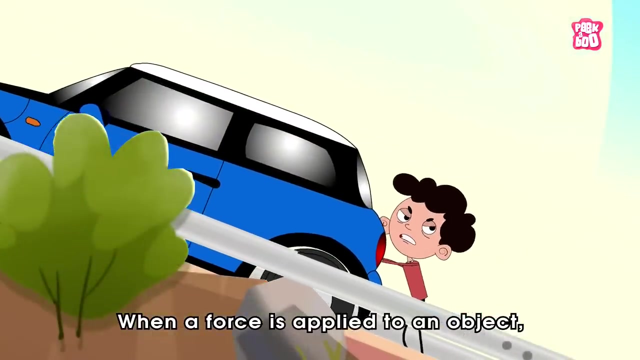 And to understand both the forces quantitatively. the force is measured in the unit Newton. But the application of force does not end the topic. In fact, it takes us to the next step of force applied, called work. When a force is applied to an object, it results in the movement of an object. 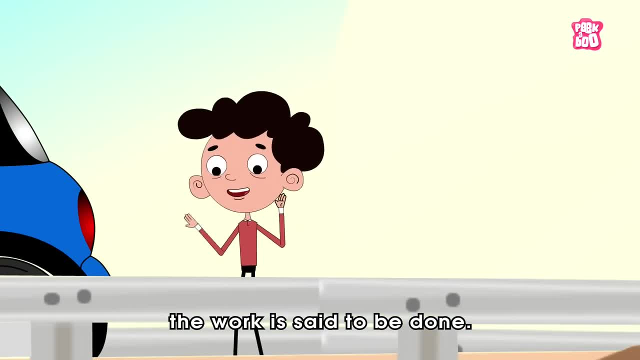 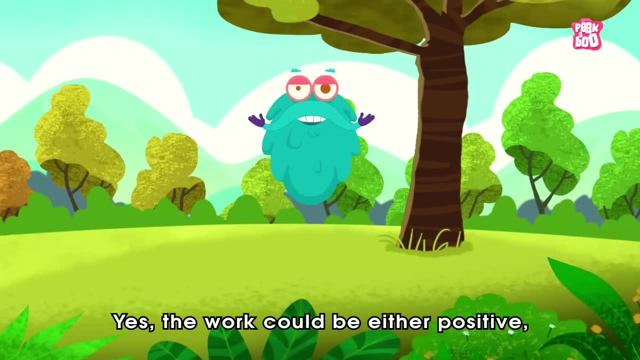 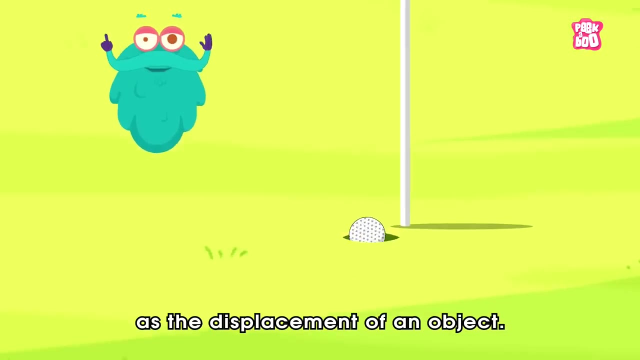 And when this happens, the work is said to be done, And even the work performed can differ in various forms. Yes, the work could be either positive, which means the force is in the same direction as the displacement of an object, Or it could be negative, indicating the displacement of an object.